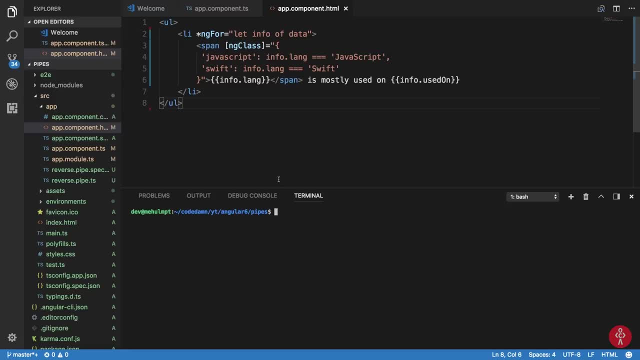 code and right here I can open my inbuilt terminal here and I can say ng generate directive. and let's just say I create a directive which is red, black and I'm just going to tell you what that means. So I wrote ng generate directive. it created me two files and updated the module. Let's just see what it updated inside our 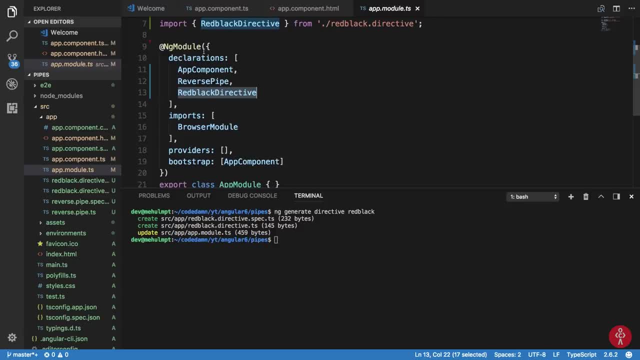 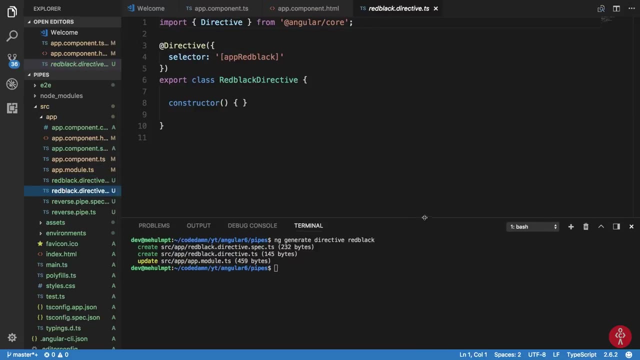 module file. You can see that it added red black directive inside declarations, right, and it has included that as well. Very nice, very nice. Now what we can do is just look at this red black directive And you can see that it has a selector of app- red black. Now what Angular does is that it prefixes your 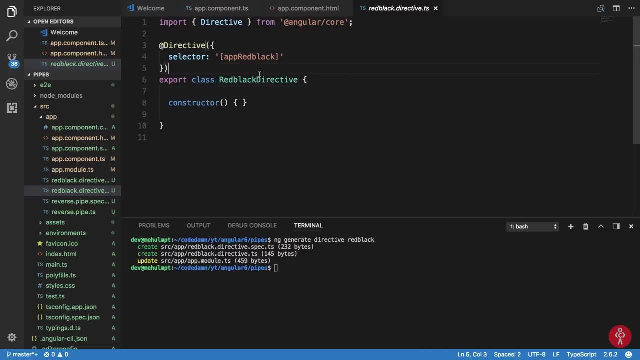 directives with something, so that you do not clash with Angular's inbuilt or some other library's inbuilt directives by mistake. So this is just a security measure. you can say from Angular team: You can change this to whatever you want, But I'm just going to keep it this way And this is basically the directive name. you need to add your. 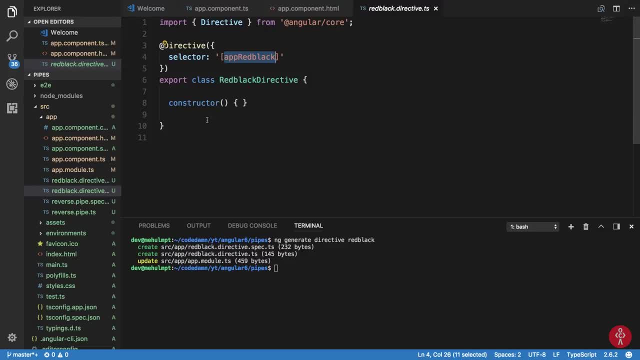 html elements in order to Let this static run. So I'm just going to go Right here And I'm going to create a paragraph. I'm going to say This paragraph: beraduya Rasheesh is a normal. And I'm going to create another one and say this paragraph: 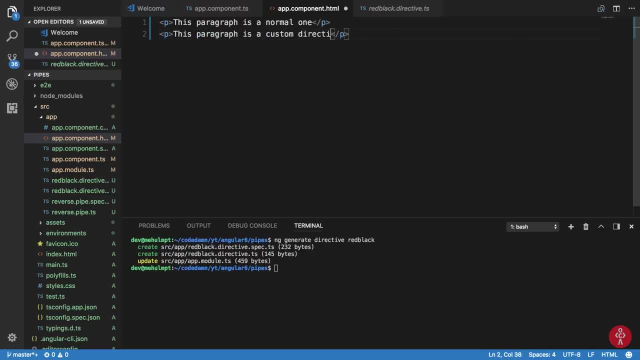 is a custom directive one, and I'm gonna add this app- red, black, dark. so now let's just code what this app red black directive would look like. okay, so the obvious thing we need to customize the HTML element we are working on is first of all, get that element right. so, right here, we do not see any way to get that. 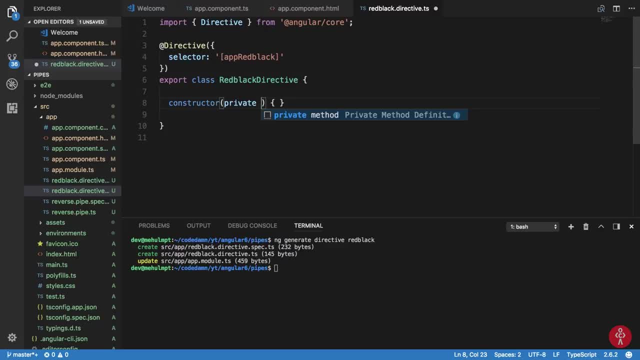 element. so what I'm gonna do is inject a dependency of that element and I'm gonna instruct angular to give a reference, give me reference to that element. so what it does is that it gets us to that particular element on which I have placed this directive. so, as a matter of fact, let's just console log this EL guy. 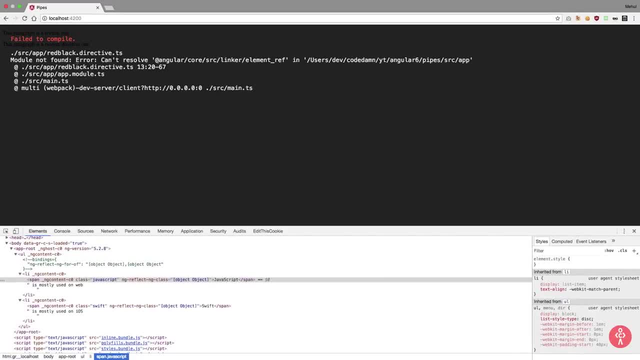 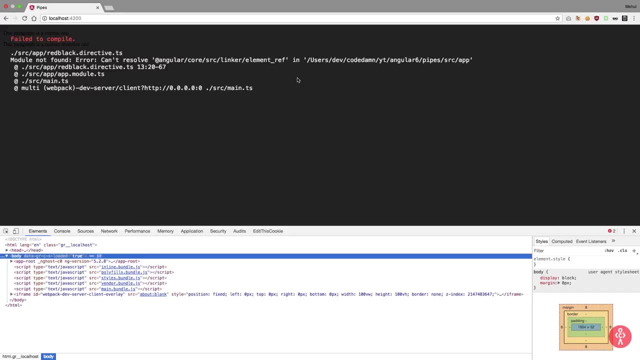 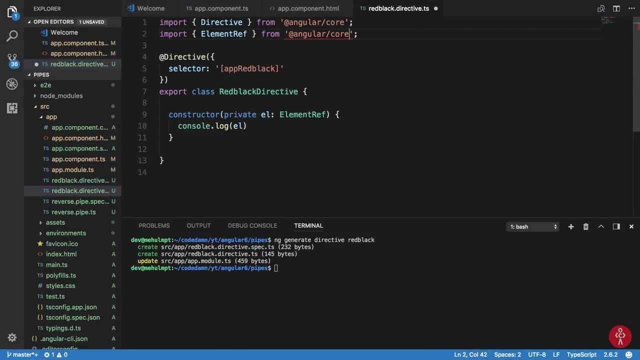 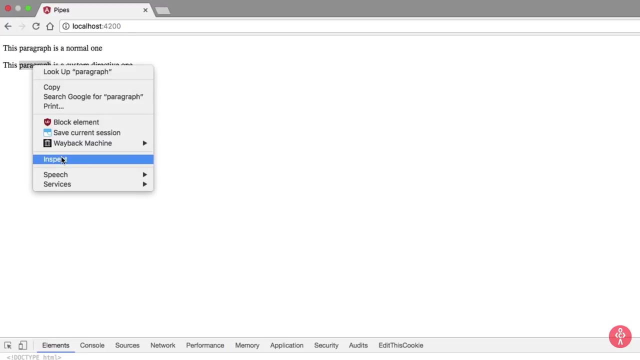 right now. so now if we go to browser and see and and actually VS code always gets this wrong. this should be just angular core right and now. if we go here, you can see that we get this as paragraph is a custom directive one, but inside console we get this element reference, so you can. 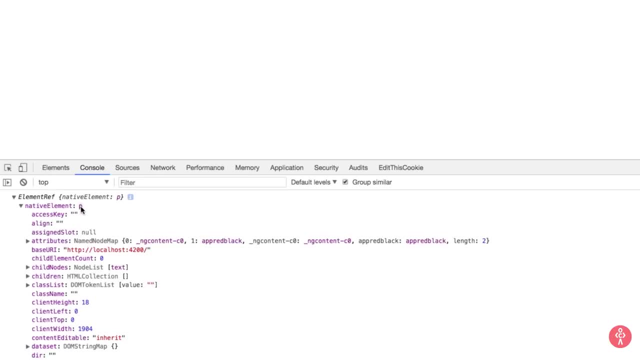 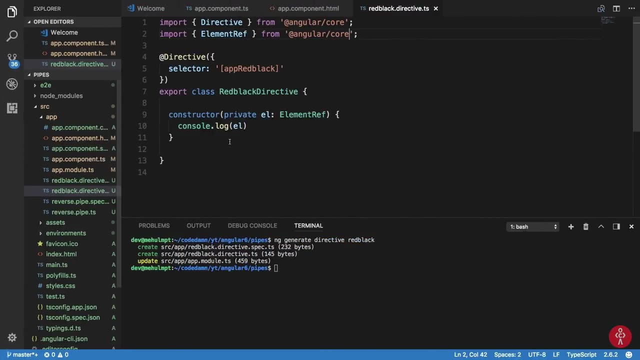 see that we get a native element reference and once we get that native element, it's the same as the one on the page, so we can mess around with that. so let's just mess around with that. I'm gonna say: EL dot native element. now this gives us access to the P tag we have on the web page. so I'm just gonna. 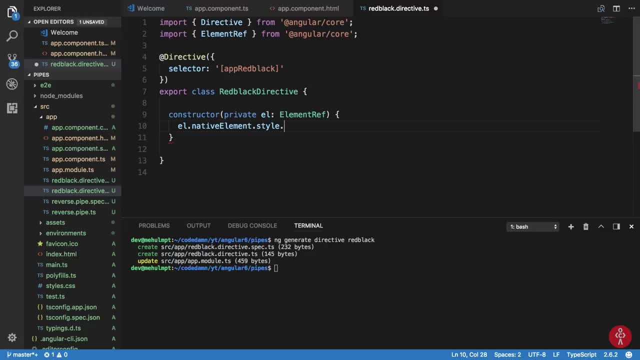 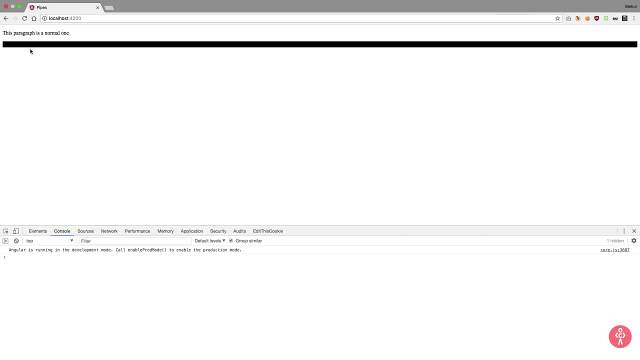 style it and say color or text color, I don't remember really. let's just assume it's text color, make it white, and I'm gonna do the same thing with the background color and make it black. let's just see, yeah, it should be actually color, or? 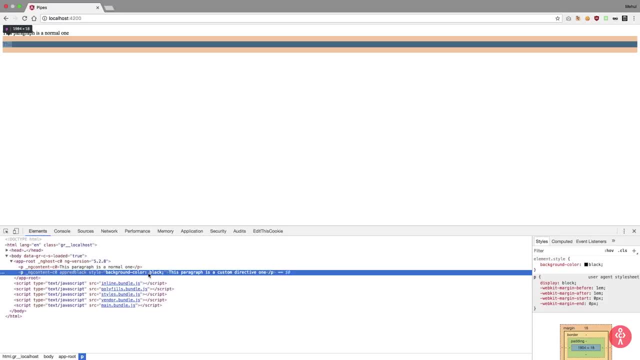 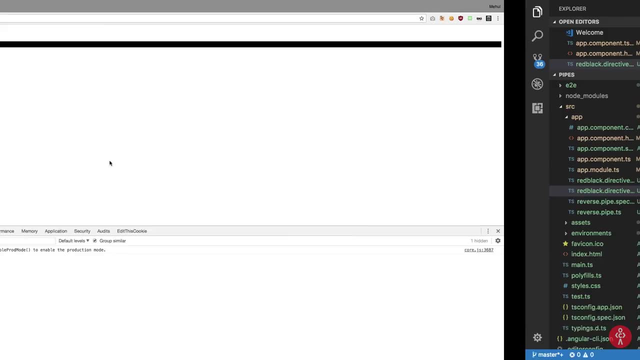 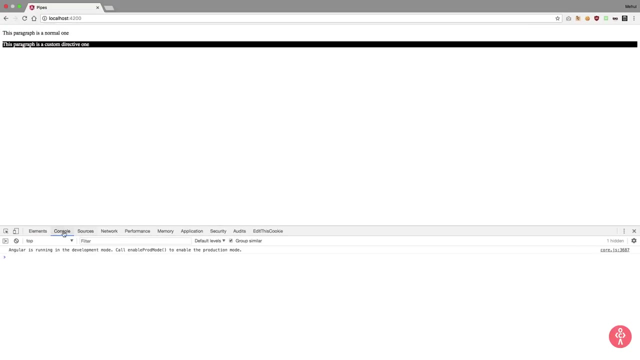 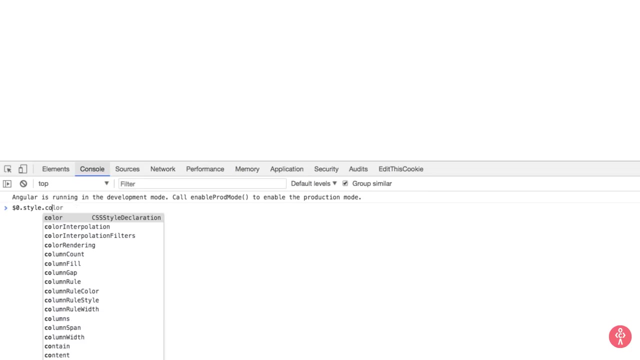 should it be? background color is black, color is white. okay, that makes it work, but I don't really remember what the property name was here. let's just take a look from here. only element or style dot color is white. style dot text born. what the hell is this? 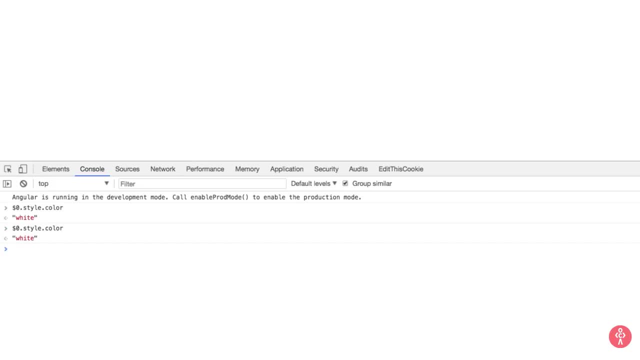 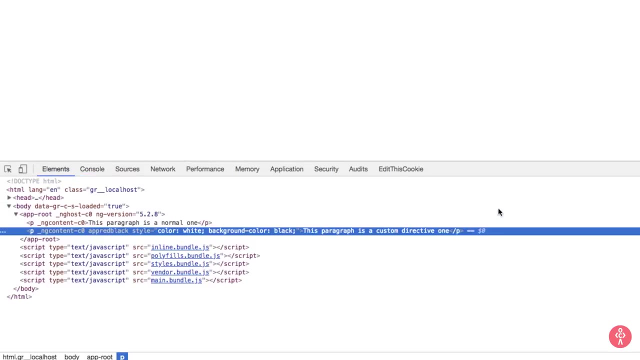 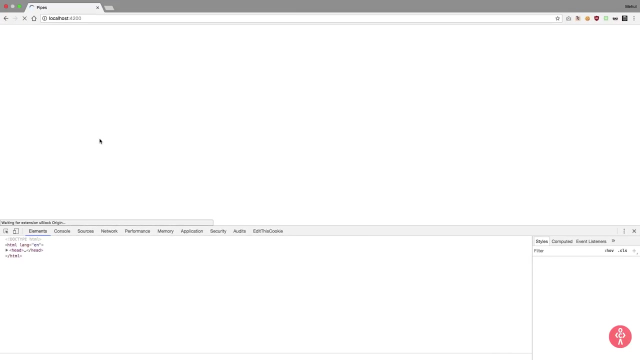 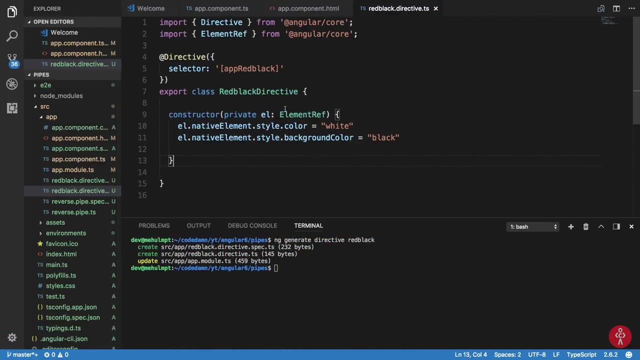 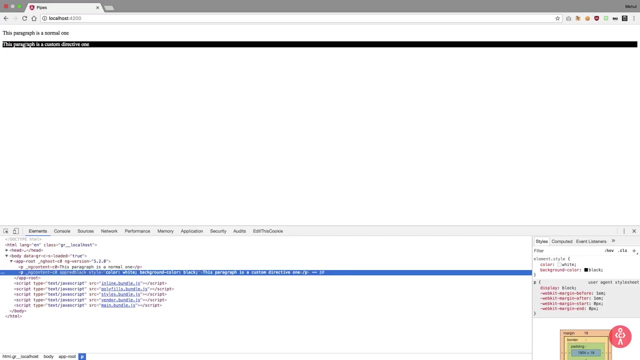 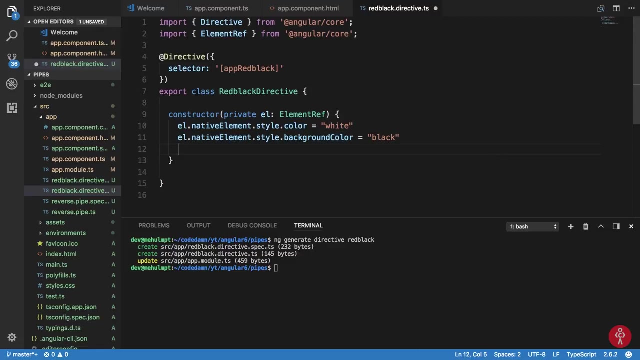 ok, so it was running some what's happening. let's just save this and reload it again. damn you angular, you were running a cached copy or something. so yeah, this works. we have a custom directive which is customized according to our needs, right? so yeah. so what I can do is basically say something. 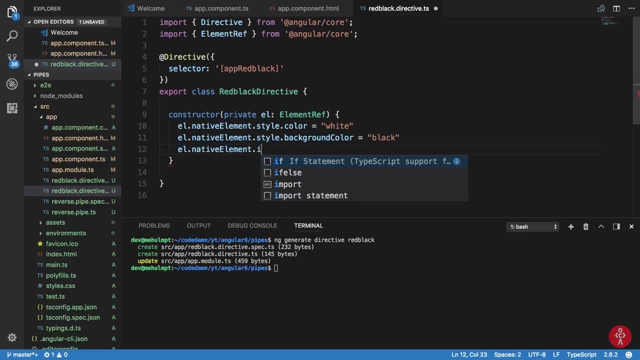 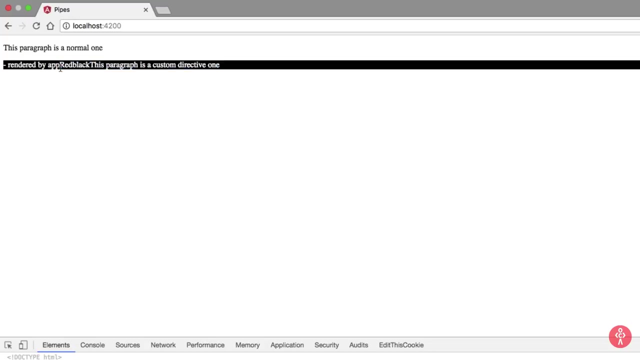 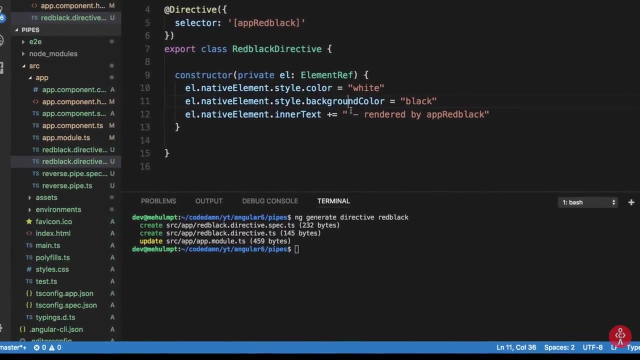 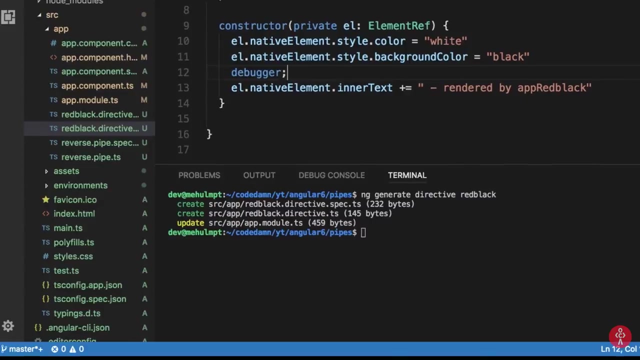 like EL dot native element, dot inner text plus equals to rendered by app red black, so you can just add a notice or something like this, or actually: okay, rendered by app red black. we get it like this, but what I want is okay, so let's just take a look if I add a debugger here. 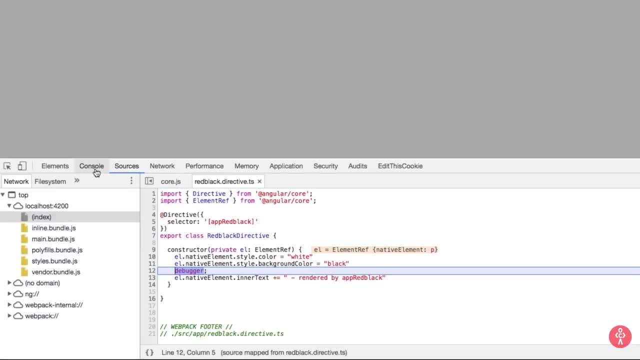 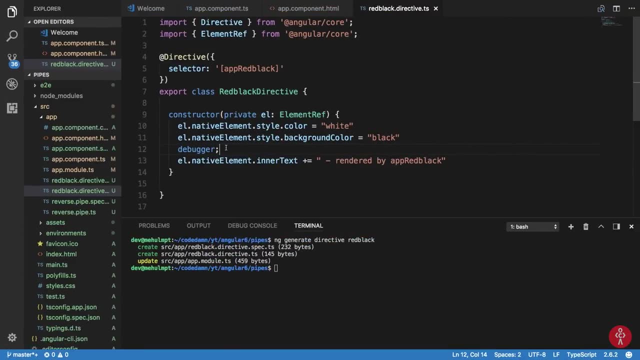 go to console, you see that this directive is called before the element is rendered. so at this time, what happens is that the directive we are, this thing we are working on, is empty, so we do not have access to whatever inside this element is. so again, you can add something like ng on in it here and 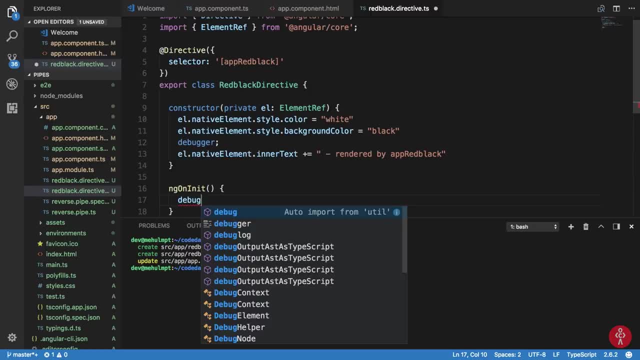 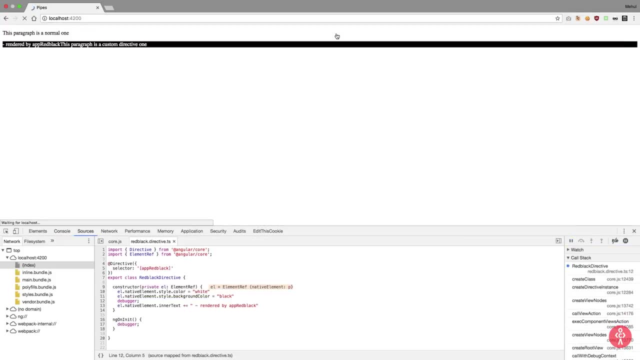 you can add something like ng on in it here, and you can add something like ng on in it here and add a debugger call. add a debugger call. add a debugger call here as well. here as well, here as well. play this thing, reload, play this one and. 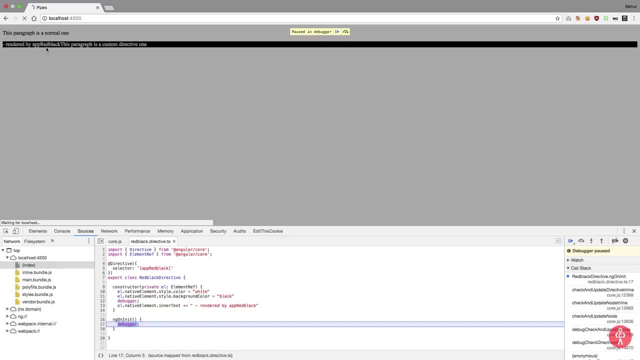 play this thing. reload, play this one and play this thing. reload, play this one. and now you can see that ng on in it is. now. you can see that ng on in it is. now. you can see that ng on in it is called after the content is rendered so. 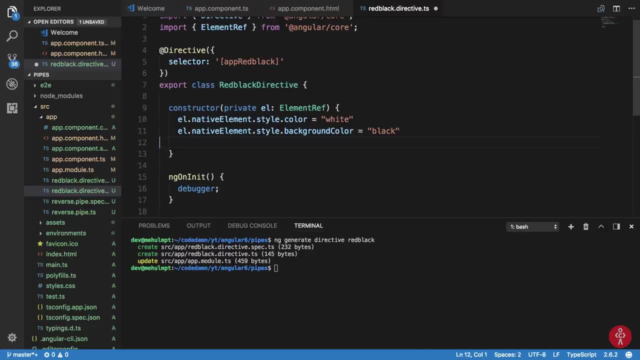 called after the content is rendered. so called after the content is rendered. so this is why messing around with content. this is why messing around with content, this is why messing around with content inside constructor would not work and you inside constructor would not work and you inside constructor would not work, and you will need to place your stuff like this: 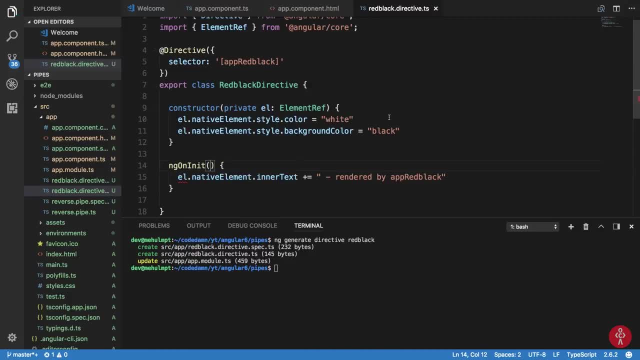 will need to place your stuff like this, will need to place your stuff like this inside your ng on in it, and we can just inside your ng on in it and we can just inside your ng on in it, and we can just create this element. create this element. 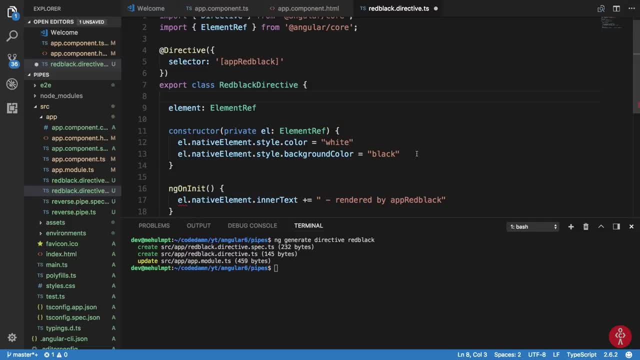 create this element as element ref. as element ref. as element ref. now. can just say this dot element is now. can just say this dot element is now. can just say this dot element is here and then inside ng on in it: i'm here. and then inside ng on in it: i'm. 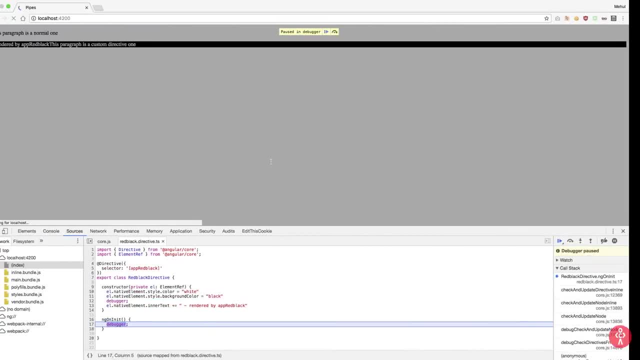 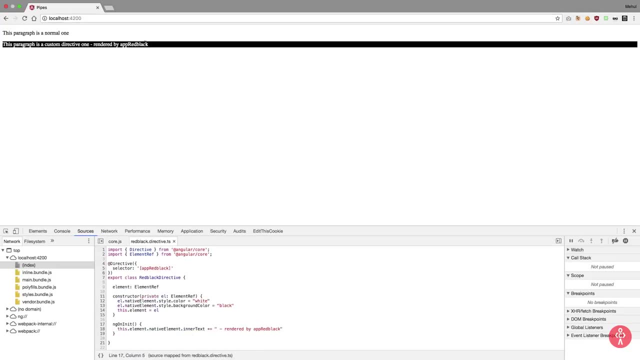 here and then inside ng on in it. i'm just gonna say this dot element, just gonna say this dot element, just gonna say this dot element: yep, hit on, play, yep, hit on, play, yep, hit on play, reload this guy, reload this guy, reload this guy, and you can see that it's now in order.